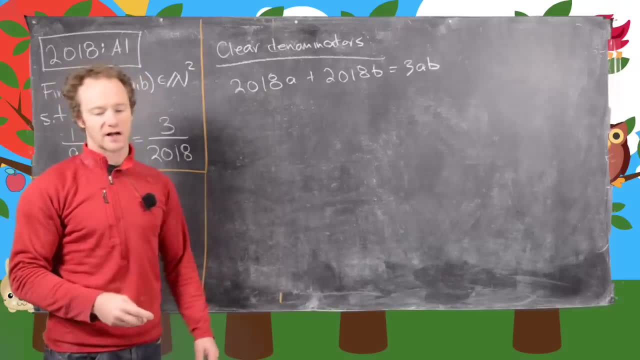 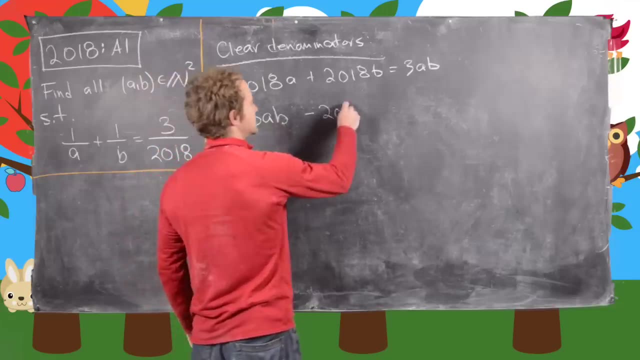 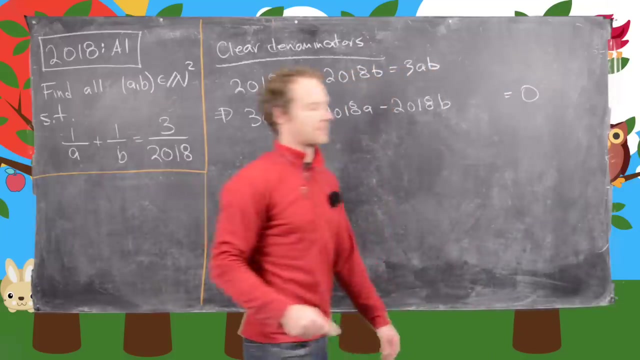 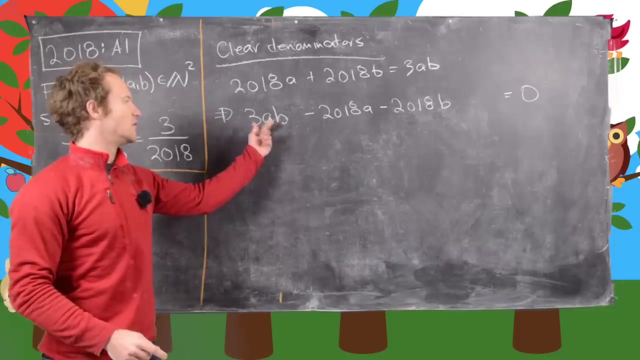 So it'll be like completing the square, but really we're just completing a product of a binomial. So, in other words, let's rewrite this as: 3AB minus 2018A minus 2018B equals 0.. Okay, so now from here, it looks like I could factor this into a binomial that starts with an A. 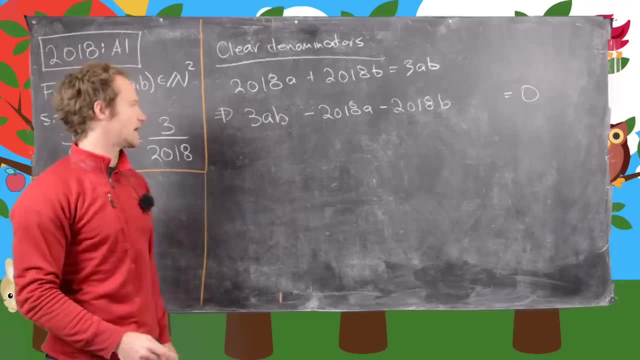 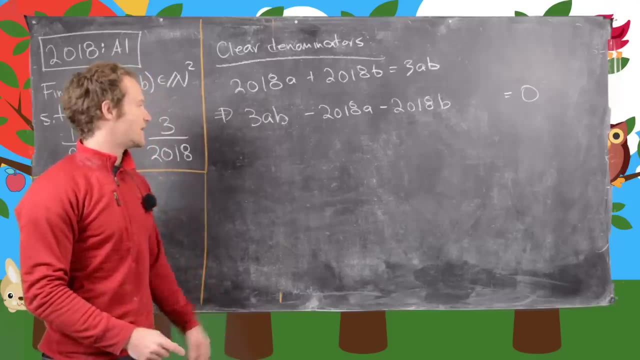 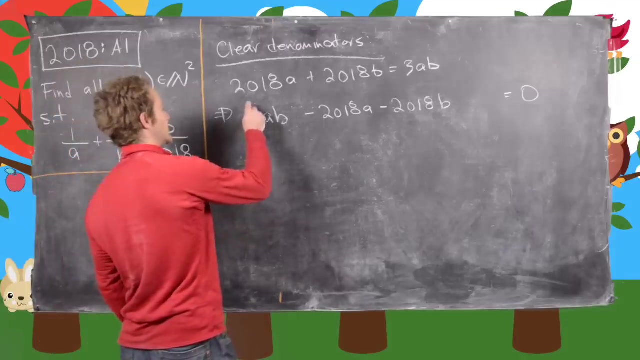 and a binomial that starts with a, B, That would multiply together to get 3AB. But it's a bit of a problem because we'd like to have a bit more symmetry in the problem than that would allow. So we can get that by replacing 3 with 9, by multiplying this whole thing by 3.. 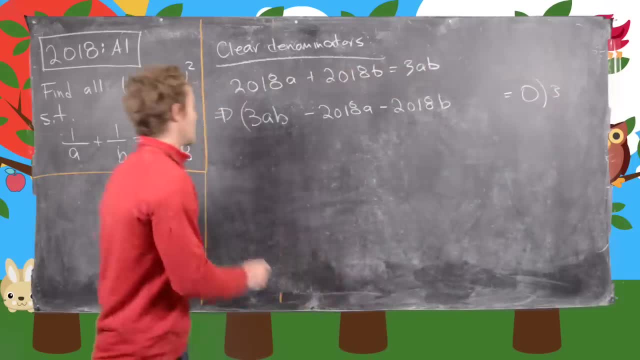 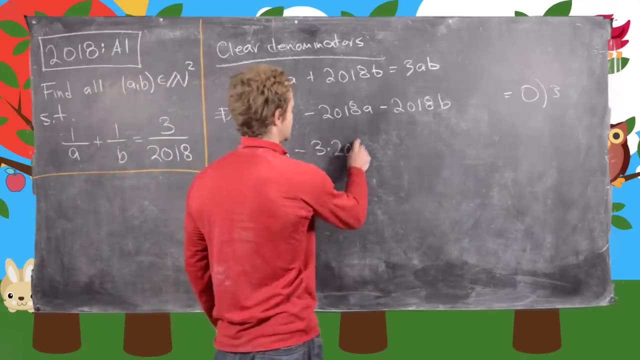 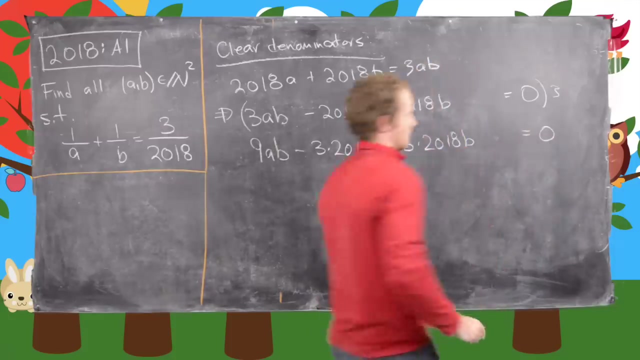 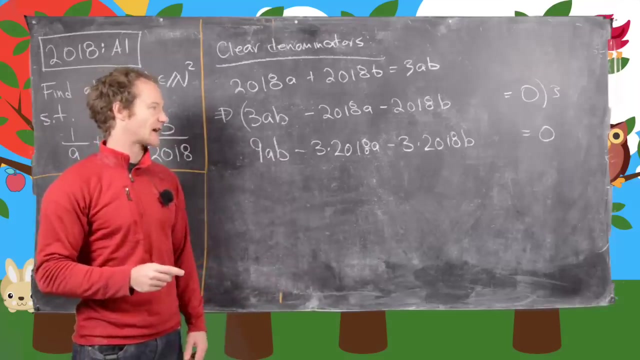 So let's multiply this whole thing by 3. And that's going to give us 9AB minus 3 times 2018A minus 3 times 2018B. Okay, Now we can go about not completing the square, but completing this into a factorable binomial on the left-hand side of the equation. 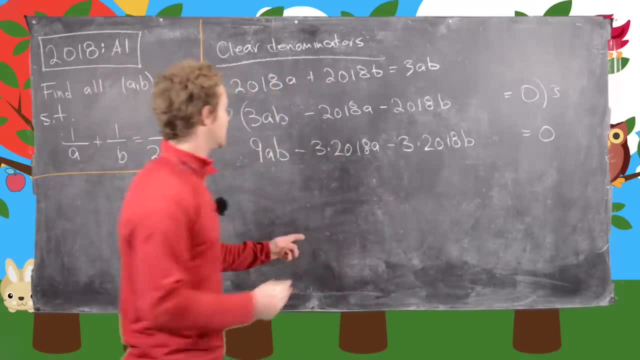 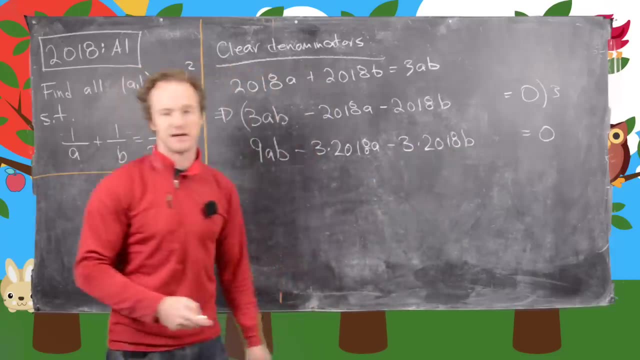 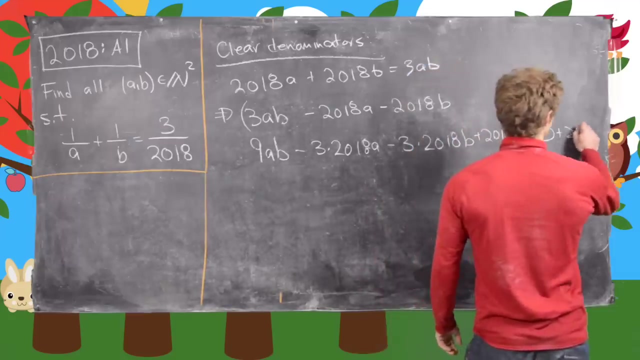 And we can do that by noticing that here we have 3 times A times 2018.. Here we have 3 times B times 2018.. So if we add 2018 squared to both sides, then we're good to go. 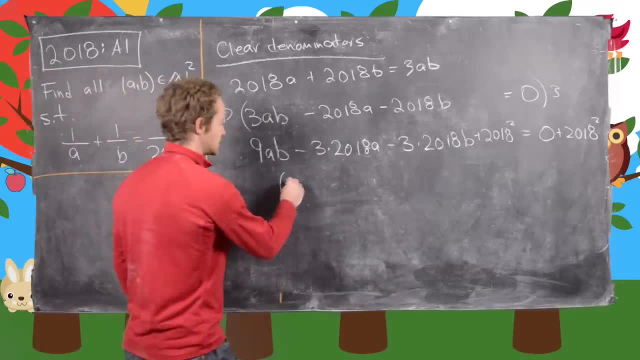 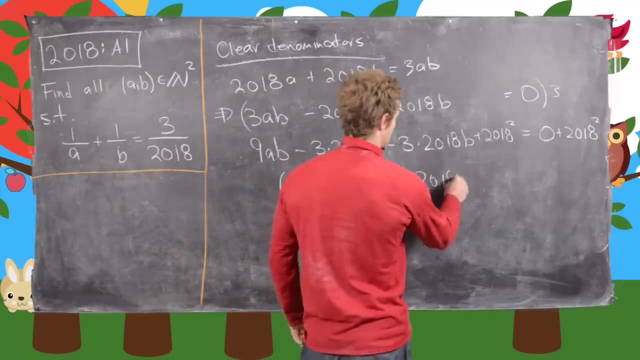 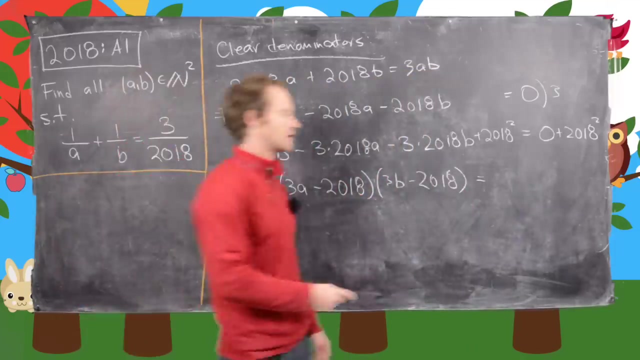 And now this left-hand side of the equation. we'll factor as follows: We'll have 3A minus 2018 times 3B minus 2018 equals 2018 squared. But I'm going to go ahead and factor that into primes because that'll be useful later. 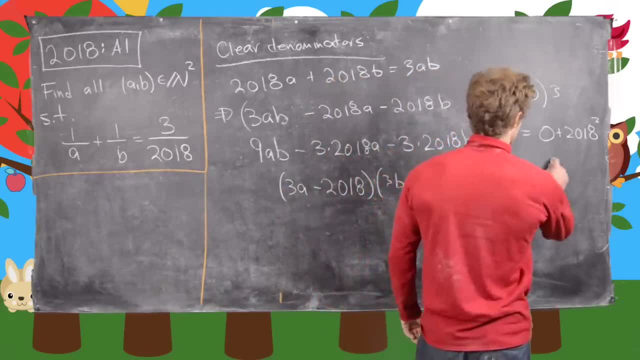 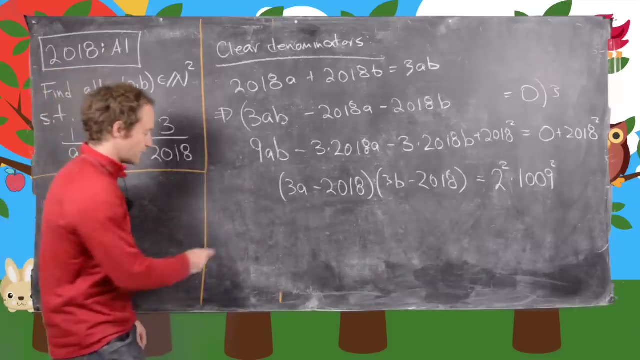 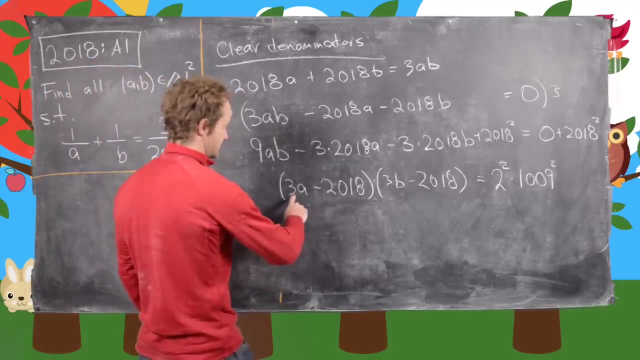 So that is 2 squared times 1009 squared. So now what we'll do is look at this whole thing. We'll look at this whole thing, mod 3.. So if we reduce this mod 3, we get the following: So notice that this bit is 1 mod 3.. 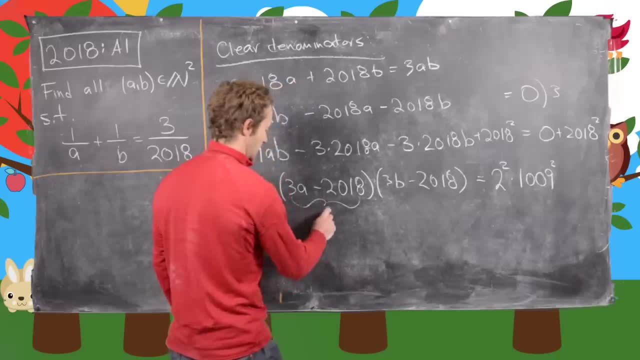 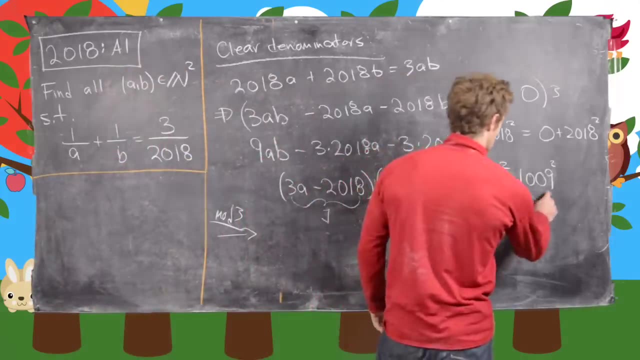 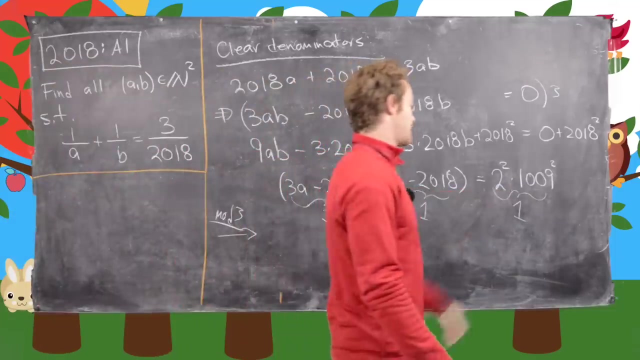 So this is 1 mod 3.. This is also 1 mod 3.. And then that over there is also clearly 1 mod 3.. So that means a good strategy here is to look for factor pairs of this right-hand side of the equation. 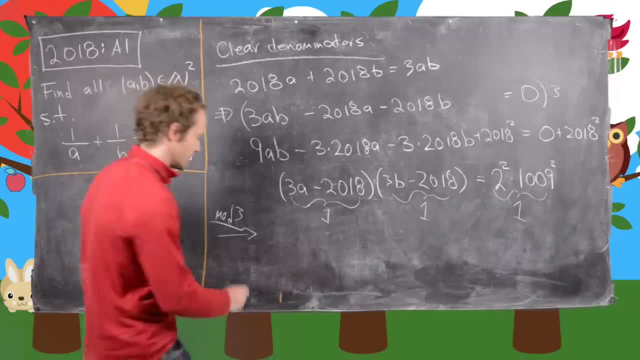 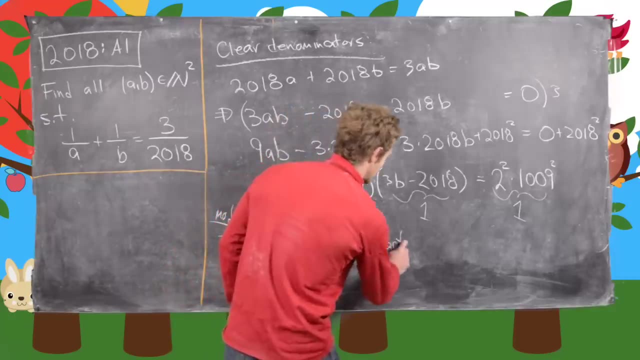 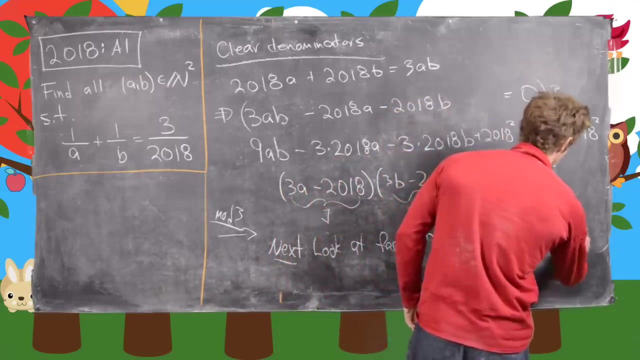 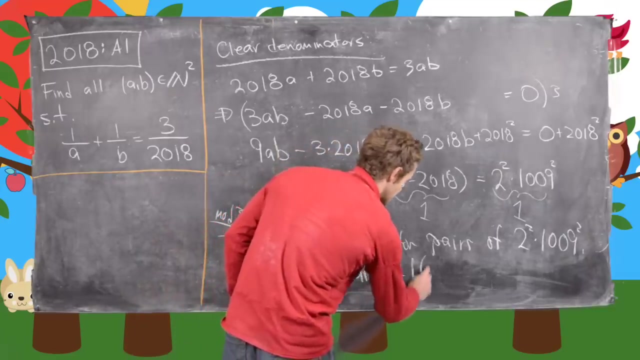 where each part of the factor pair is 1 mod 3.. So, in other words, our next step is to look at factor pairs of 2 squared times 1009 squared, where both are congruent to 1 mod 3.. Okay, good. 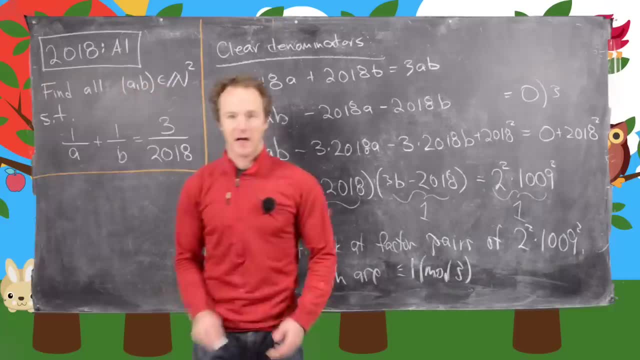 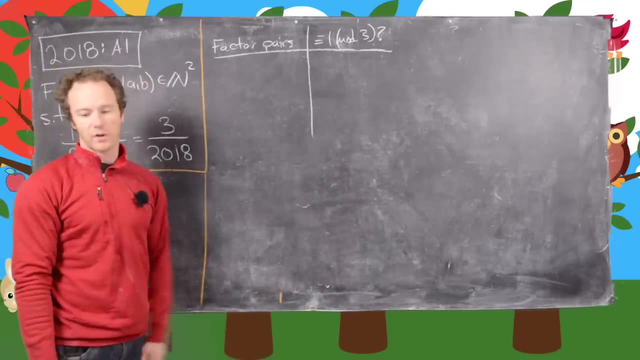 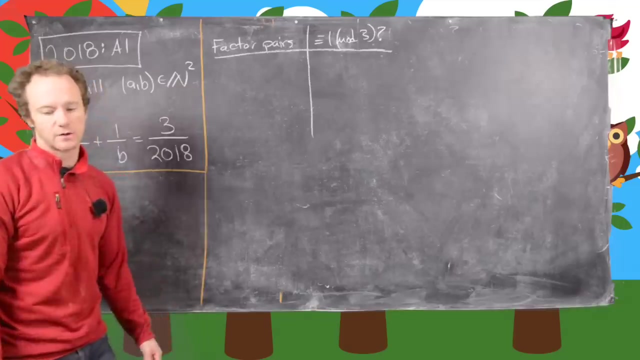 So I'll clean up the board and then we'll move to the next step. Okay, So let's make a little chart of the factor pairs for the number we're interested in and then answer the question: which of those factor pairs have the property that both are congruent? 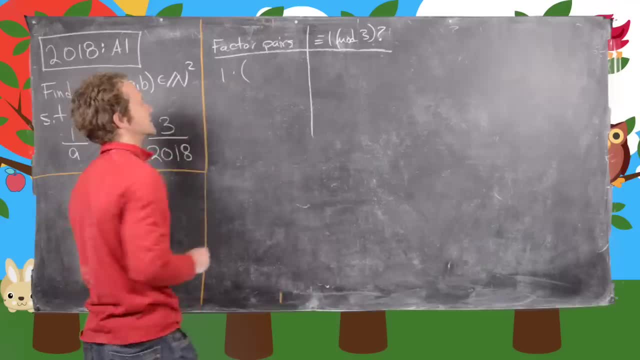 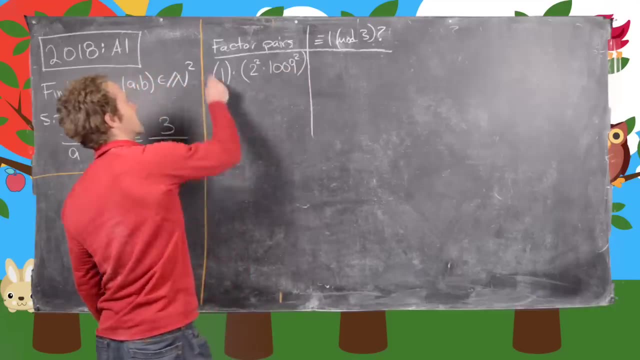 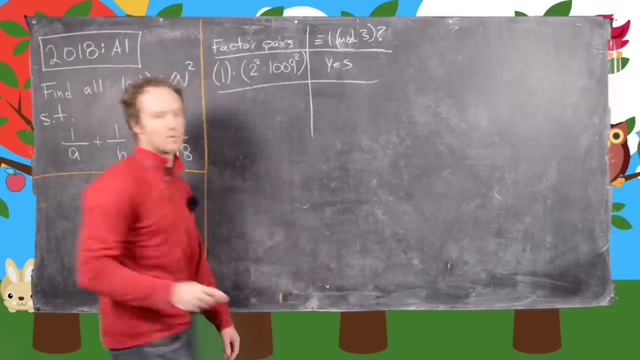 to 1 mod 3?? So our first factor pair is going to be 1 times 2 squared times 1009 squared. So there we have. This is one part of the pair. This is the other part of the pair And in this case, yes, they are both congruent to 1 mod 3.. 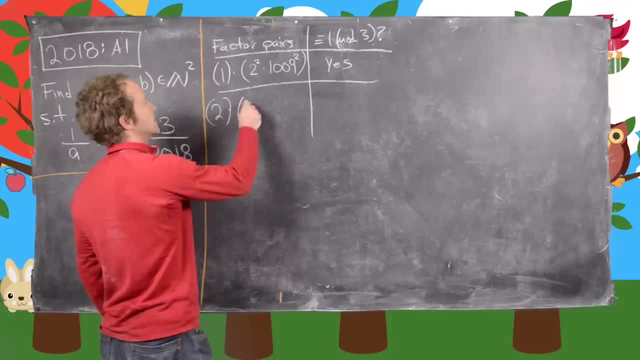 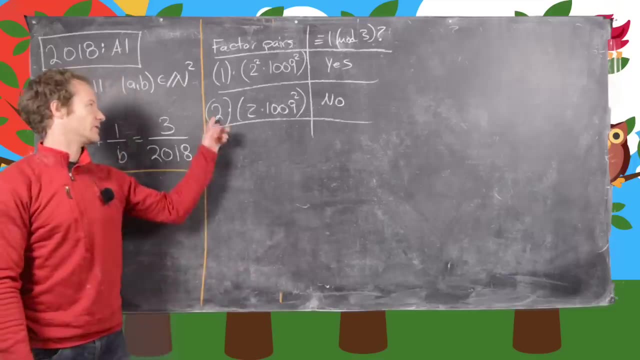 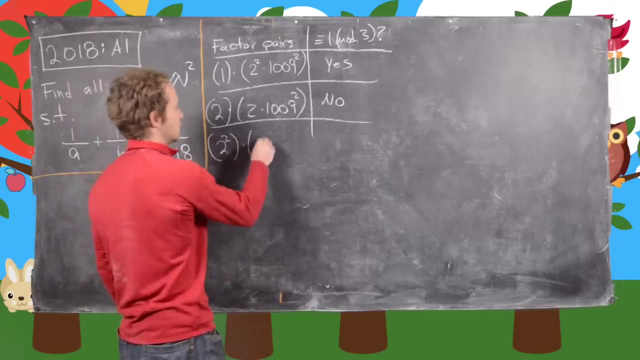 Now the next one will be 2 times 2 times 1009 squared. But in that case, no, they are not both congruent to 1 mod 3. We have to throw that one away, Okay? And then the next one will be 2 squared times 1009 squared. 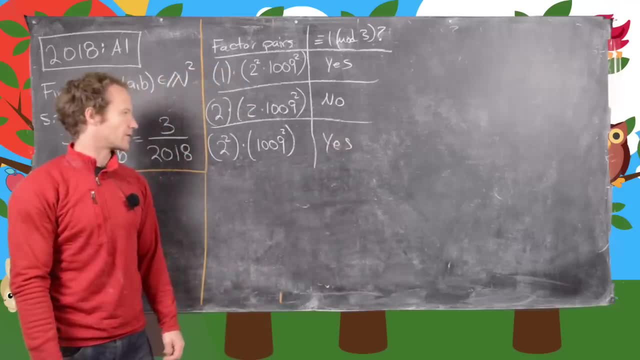 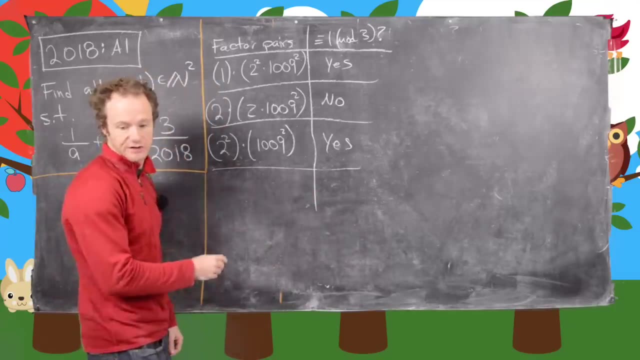 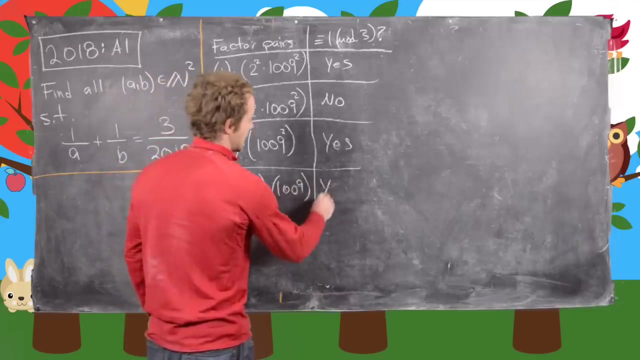 And the answer to this is again yes. They are both congruent to 1 mod 3.. Okay, And then we've got one more. So we've got 2 squared times 1009 and then 1009.. And again yes. 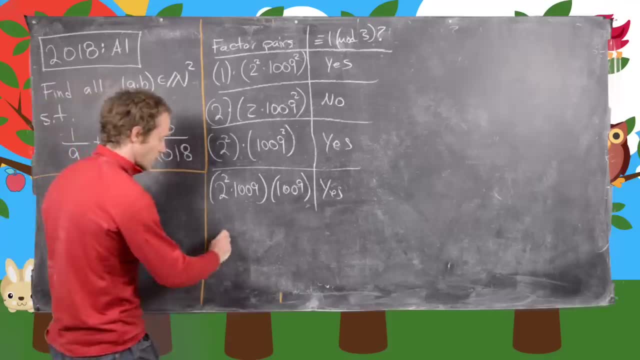 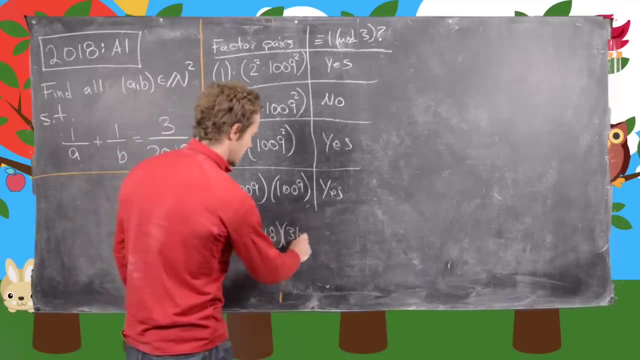 These are both congruent to 1 mod 3. And so let's just recall that we're looking at the equation 3A minus 2018, 3B minus 2018, and 3B minus 2018.. Okay, 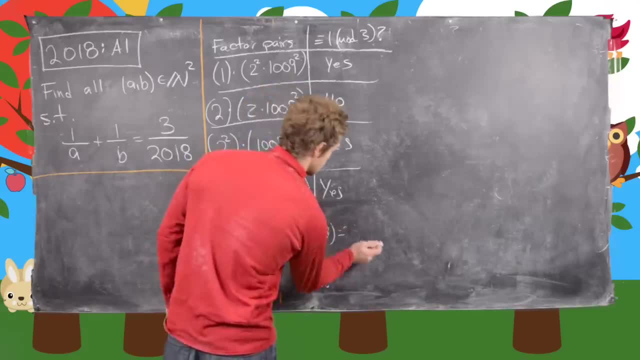 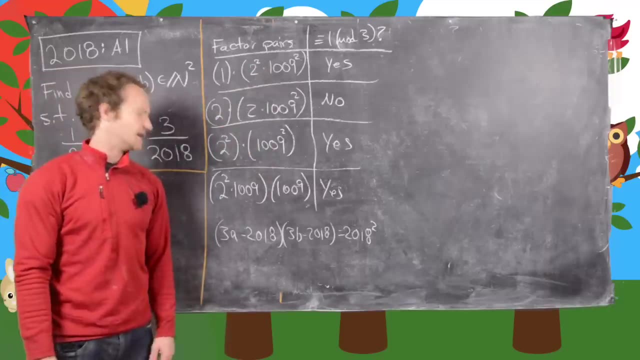 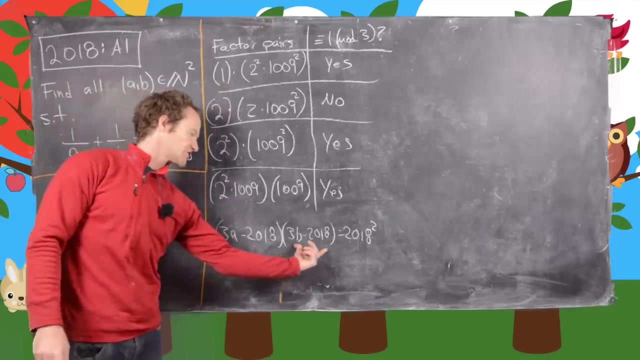 So let's just recall that we're looking at the equation 3A minus 2018 equals 2018 squared, which is 2 squared times 1009 squared, And so what we'll do is we'll assign each part of these factor pairs to each one of: 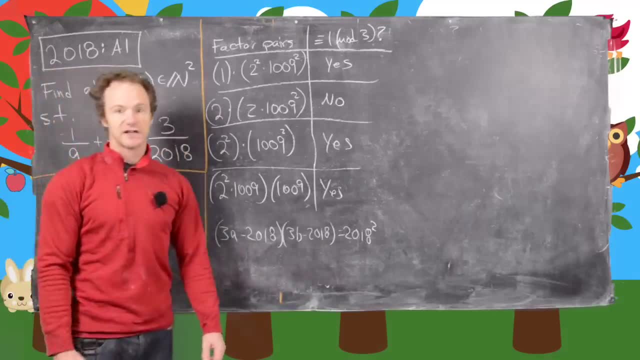 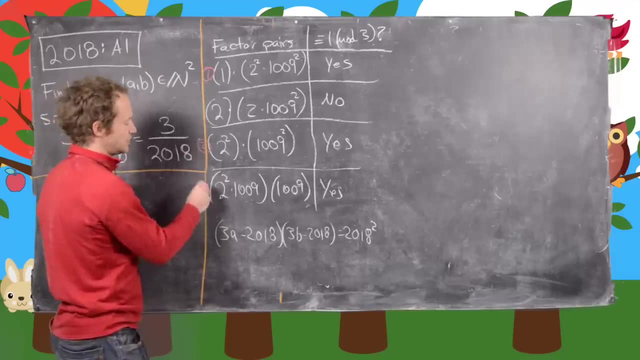 these binomials and we'll solve for A or B. So let's enumerate these. So, since this one is good, let's call it 1.. Since this one is good, let's call it 2.. And since this one is good, let's call it 3.. 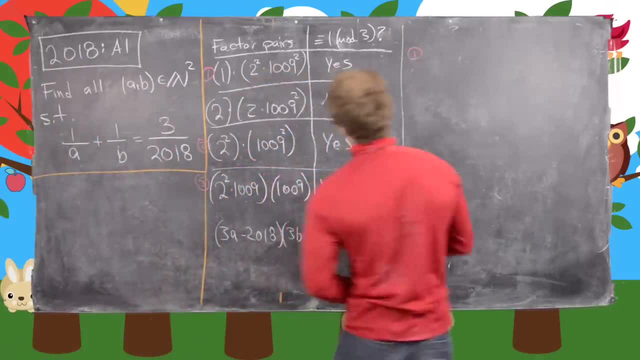 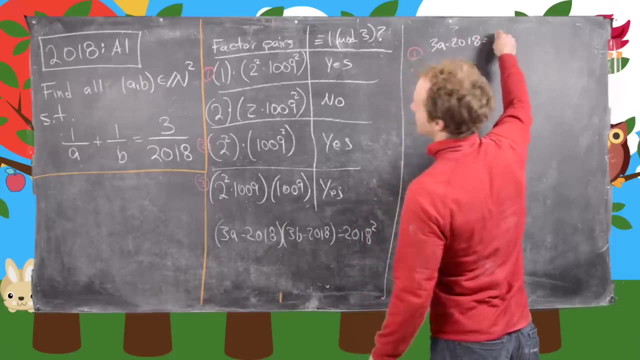 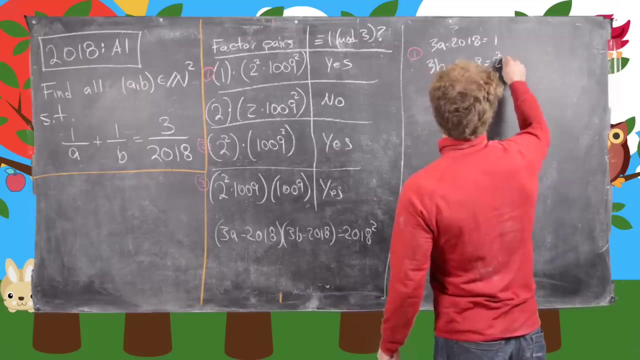 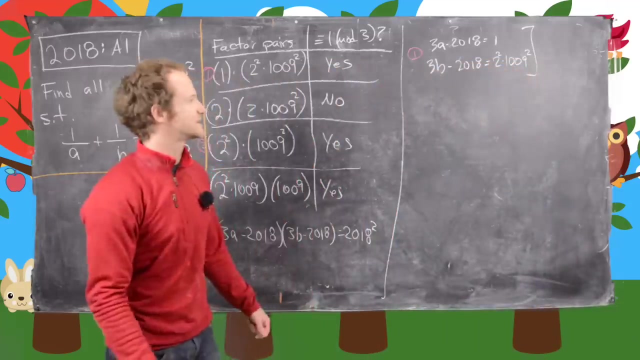 And so now let's see what we get from 1.. So what we'll have is 3A minus 2018 equals 1. And 3B minus 2018 equals 2 squared times 1009 squared. Good, So I'll just jump to the solution. 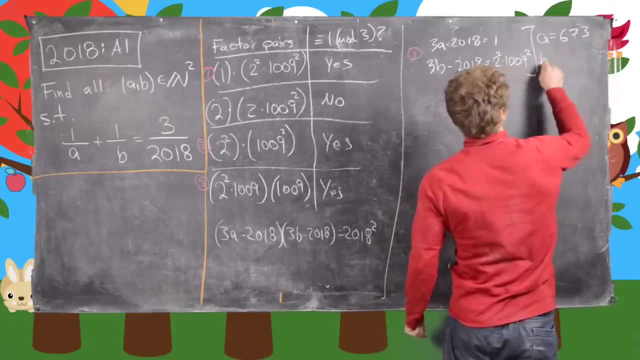 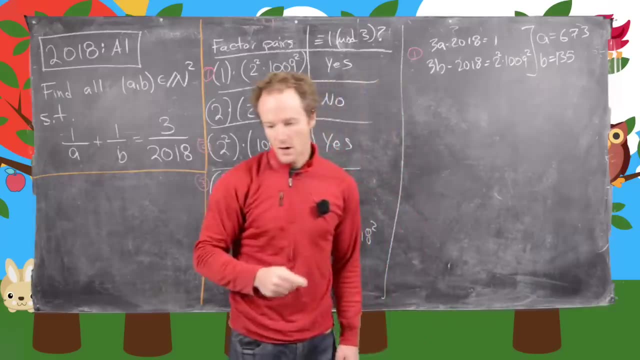 This means A is 3A minus 2018.. Okay, This means B is 673 and B is equal to 1, 3, 5, 4, 1, 1, 4, 4, 1, 1, 4.. 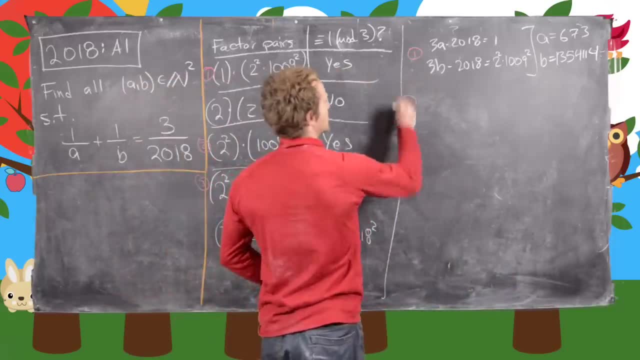 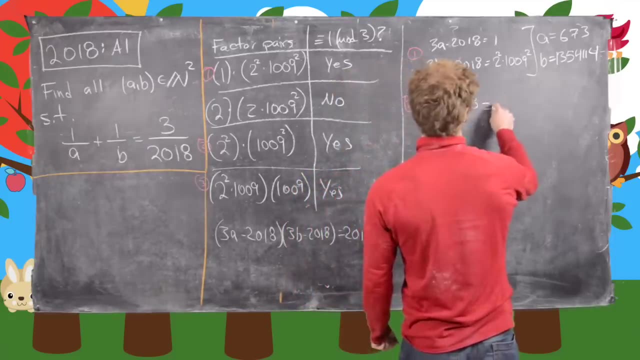 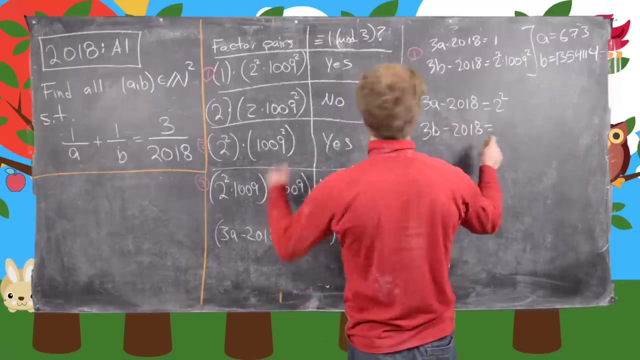 Okay, Now let's go with the second one. So we have 3A minus 2018 equals 2 squared, And then 3B minus 2018 equals 1.. So we have 3A minus 2018 equals 1, 09 squared. 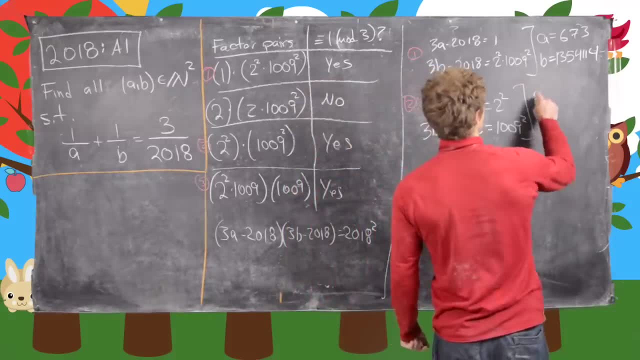 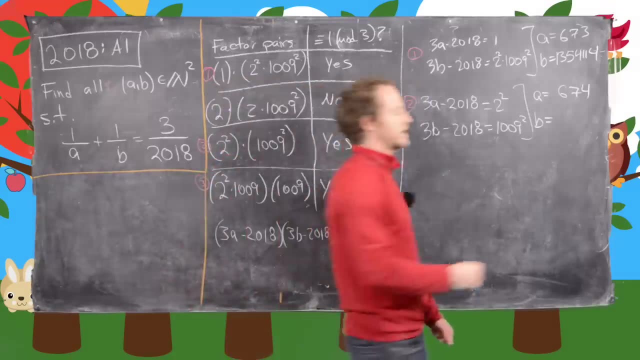 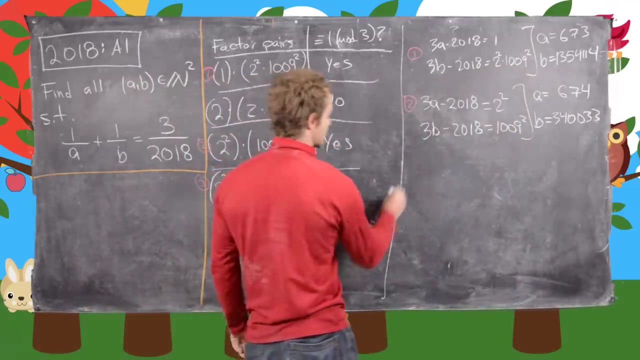 Okay. So let's see what we get there Here. we get A equals 674 and we get B equals 330,033.. Okay, And then we've got one more equation, So three. So we have 3A minus 2018 equals 3,013.. 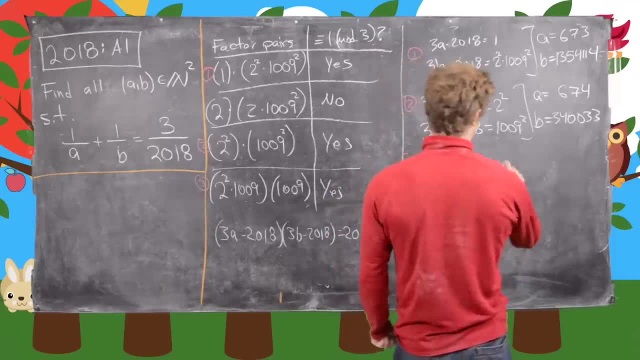 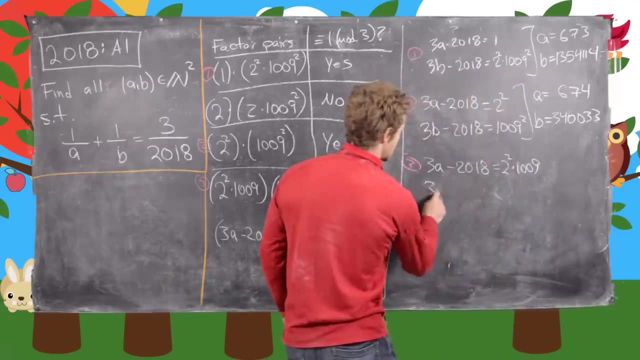 Okay, And then we've got one more equation, So three. So we have: 3A minus 2018 equals 3,010.. 2 squared times 1009, and 3B minus 2018 equals 1009.. 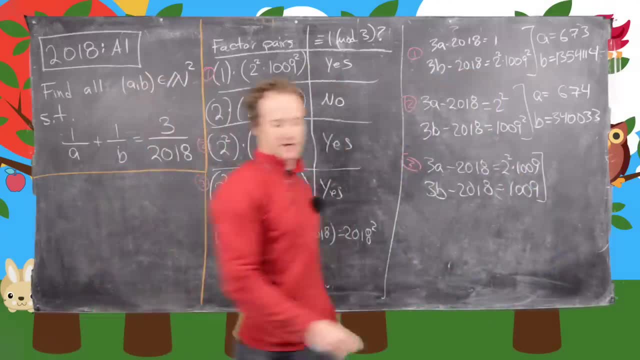 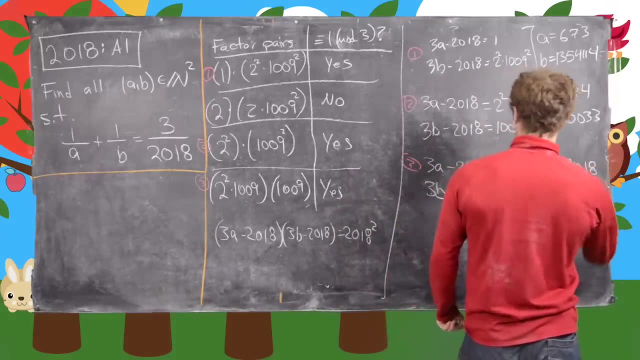 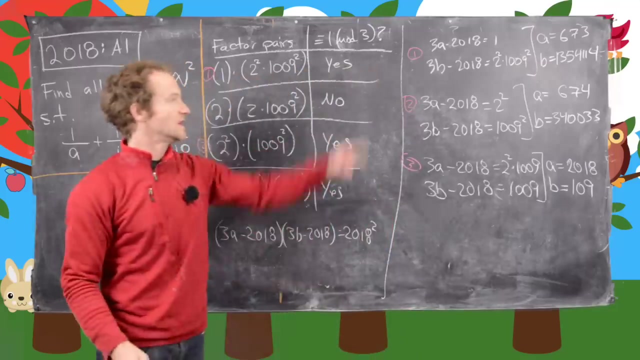 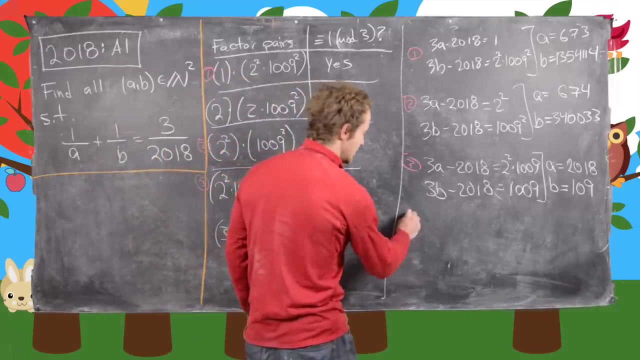 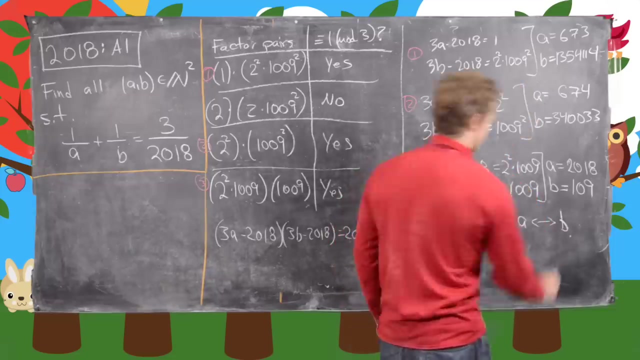 And so let's see what solution does that give us? That gives us A equals 2018, and B is going to be 1009.. So those are all ordered pairs A and B that will satisfy this if we include so, plus all swaps A with B.